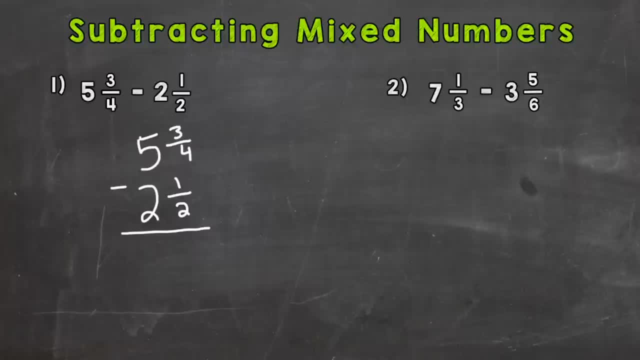 to be our common denominator For a four and a two- Hopefully you're thinking four- so let's rename these mixed numbers. Well, five and three-fourths already has a denominator of four, so we can keep it as is Now. two and a half, though we're going to need to rename. So 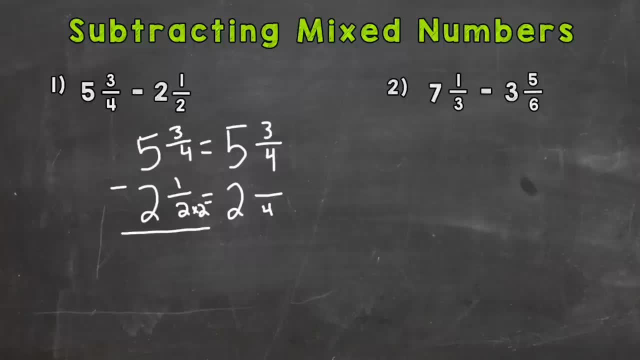 let's think two times two gives me that denominator of four, So I need to do the same thing to the top In order to properly rename. So we would do: one times two is two. Now we have our problem rewritten with a common denominator. Now subtract the fractional. 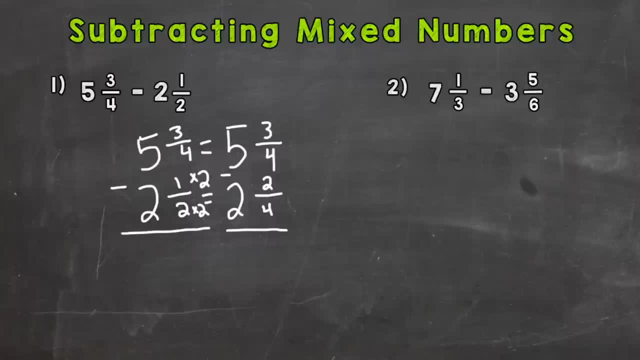 parts and then the whole number part. So three-fourths minus two-fourths. Well, three minus two is one. Keep our denominator of four the same and then do five minus two, Which gives us three. Always look to see if the answer can be simplified. the. 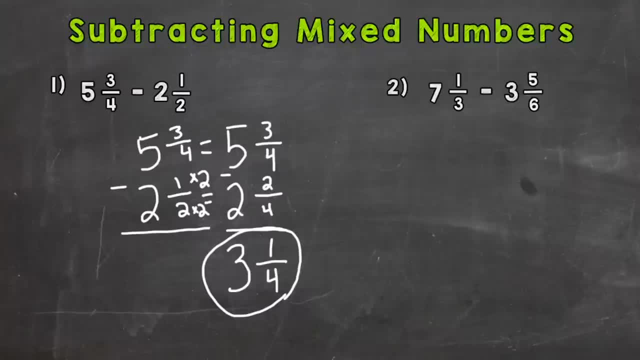 fractional part One-fourths. One-fourth is in lowest terms. so we are done. The solution or answer to number one is three and one-fourth. Let's take a look at number two. Let's rewrite the problem vertically, Which means up and down Seven. 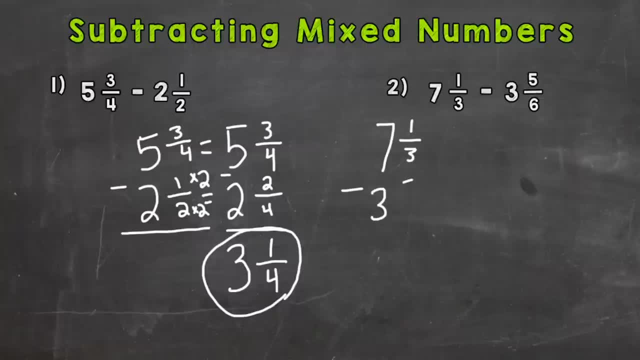 and one-third minus three And five-sixths. Alright, Let's do the fractional part first. We do not have a common denominator, So we will need to rename with a common denominator. So a three and a six, Let's think. Hopefully we're thinking a common denominator of six, So seven and. 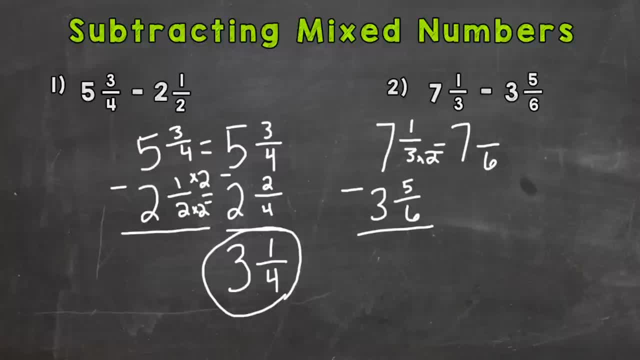 how many sixths? Well, three times two is six. One times two is two minus three. Five-sixths already has a denominator of six. So there is our rewritten problem. So let's subtract the fractional part Two-sixths minus five-sixths. Well, we can't do that. 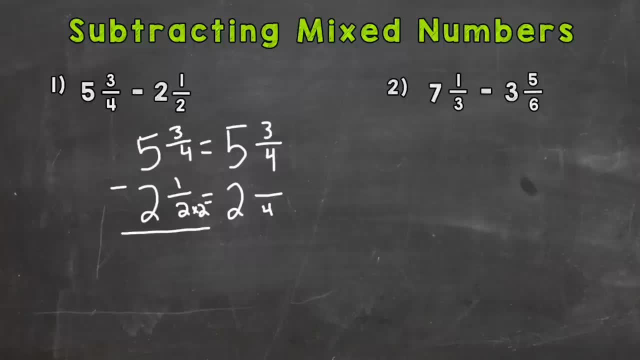 let's think two times two gives me that denominator of four, So I need to do the same thing to the top In order to properly rename. So we would do: one times two is two. Now we have our problem rewritten with a common denominator. Now subtract the fractional. 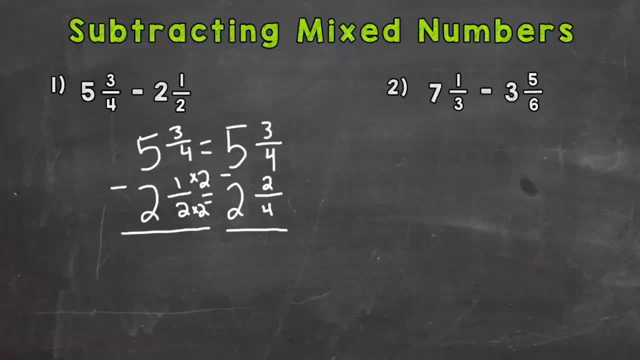 parts and then the whole number part. So three-fourths minus two-fourths. Well, three minus two is one. Keep our denominator of four the same and then do five minus two, Which gives us three. Always look to see if the answer can be simplified. the. 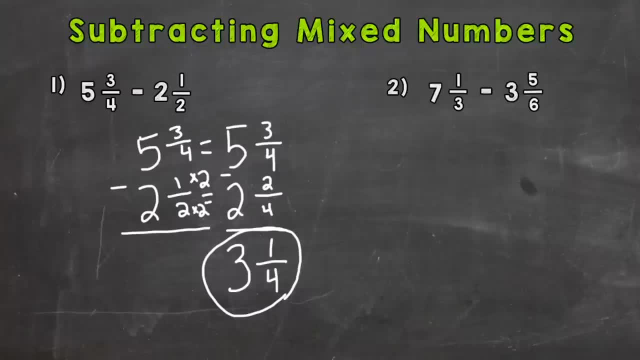 fractional part One-fourths. One-fourth is in lowest terms. so we are done. The solution or answer to number one is three and one-fourth. Let's take a look at number two. Let's rewrite the problem vertically, Which means up and down Seven. 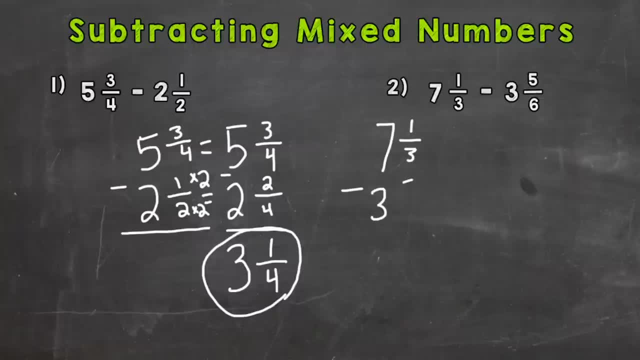 and one-third minus three And five-sixths. Alright, Let's do the fractional part first. We do not have a common denominator, So we will need to rename with a common denominator. So a three and a six, Let's think. Hopefully we're thinking a common denominator of six, So seven and. 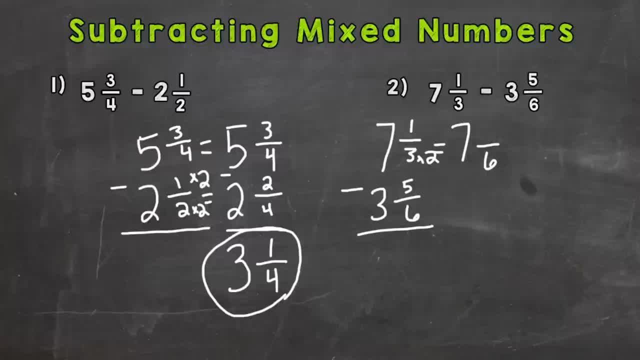 how many sixths? Well, three times two is six. One times two is two Minus three. Five-sixths already has a denominator of six. So there is our rewritten problem. So let's subtract the fractional part Two-sixths minus five-sixths. 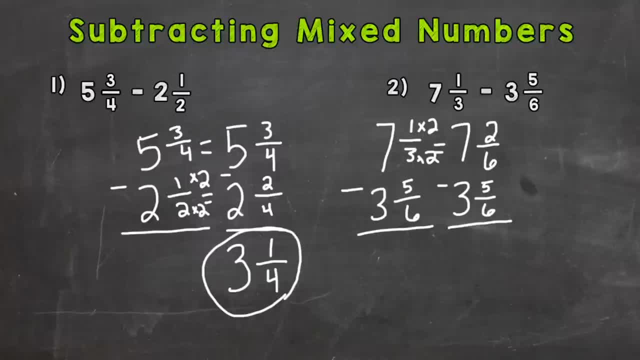 Well, we can't do that because we cannot do two minus five. So, just like a whole number subtraction problem, we need to borrow to be able to do the fractional part of this problem. So how you do that with mixed numbers, we're going to borrow one. 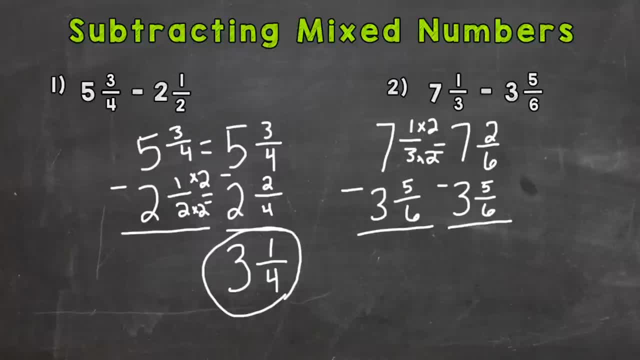 because we cannot do two minus five. So, just like a whole number subtraction problem, We need to borrow to be able to do the fractional part of this problem. So how you do that with mixed numbers, We're going to borrow one from this seven. 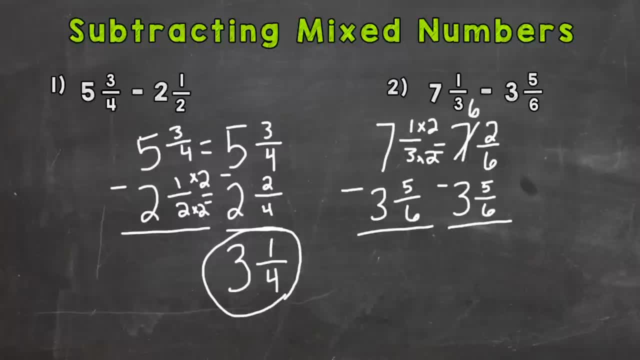 And it's going to turn to a six And we're going to add one whole to that two-sixths. Now I'm going to write one whole as six over six, So I can add it to that fractional part. They need a common denominator in order to add that whole there. 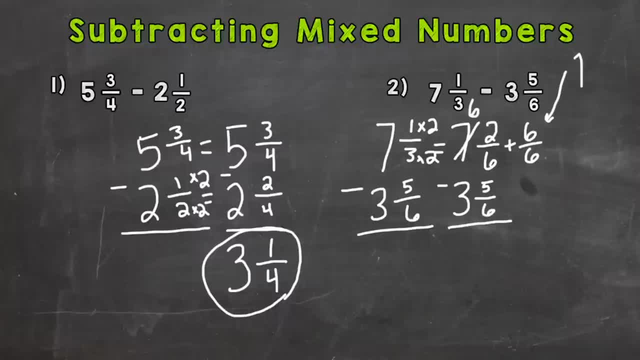 So again, 6 over 6 is 1 whole. I just put it with a denominator of 6.. So now we have 6 wholes, right, And then 2 plus 6 is 8.. Keep my denominator of 6.. 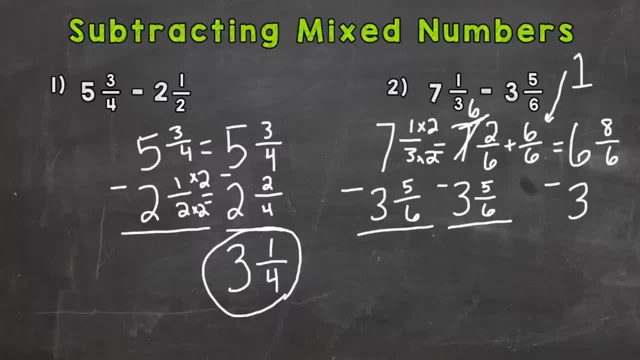 Subtract 3 and 5 sixths. Now we can do 8 minus 5 is 3.. Keep my denominator of 6.. And then we have 6 minus 3 is 3.. Check to see if we can simplify the fractional part. 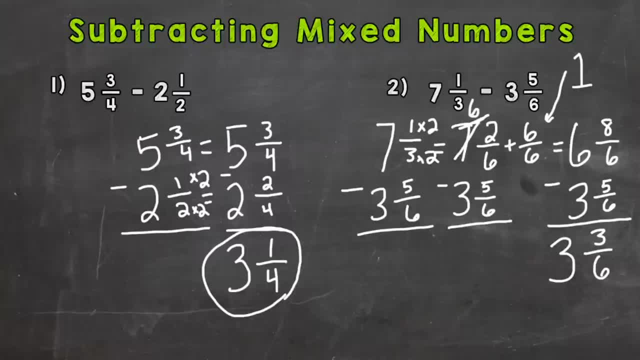 And we can. A common factor between 3 and 6 is 3.. So I can divide By 3 to get the fractional part in lowest terms, And this actually turns out to be 3 and a half. That would be our final answer there. 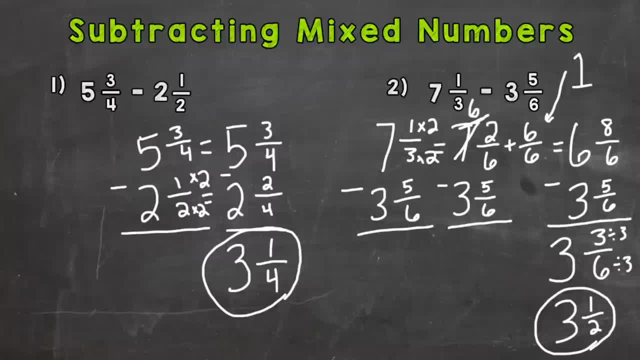 So there you have it. There's how you subtract mixed numbers. Rewrite the problem vertically. See if you need a common denominator Rename. if you do, Then go ahead and subtract the fractional part, Then the whole number part. Thanks So much for watching. 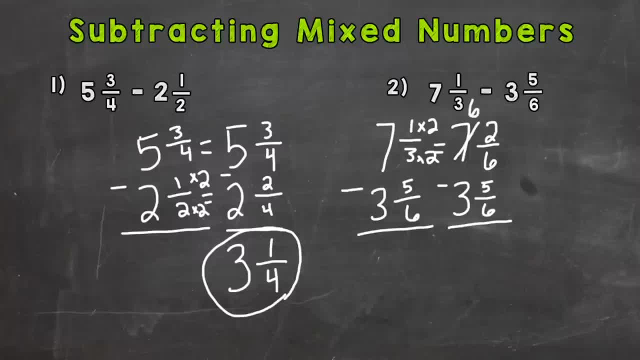 from this seven And it's going to turn to a six And we're going to add one whole to that two-sixths. Now I'm going to write one whole as six over six, So I can add it to two-sixths. 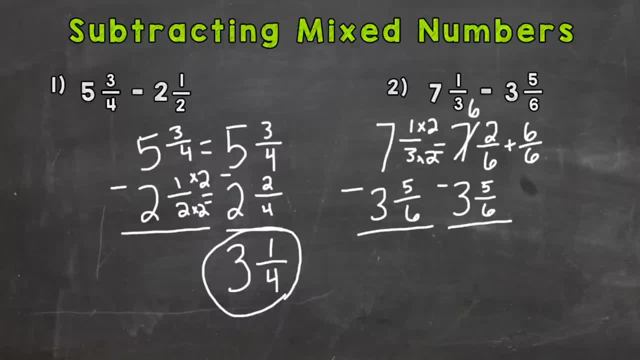 So I'm going to add one whole to that fractional part. They need a common denominator in order to add that whole there. So again, six over six is one whole. I just put it with a denominator of six. So now we have six wholes, right? And then 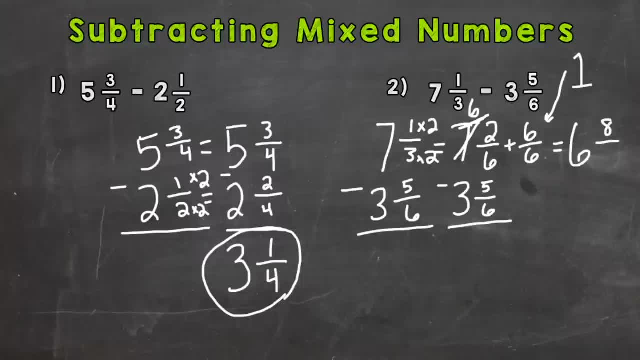 two plus six is eight. Keep my denominator of six, Subtract three and subtract two And five-sixths. Now we could do: eight minus five is three. Keep my denominator of six, And then we have: six minus three is three. Check to see if we can simplify. 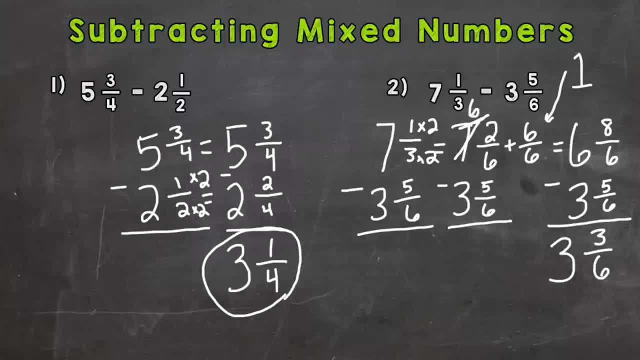 the fractional part, And we can. A common factor between three and six is three, So I can divide by three to get the fractional part, And then I can subtract the fractional part And then I can subtract the whole number part. I can subtract the whole number part. 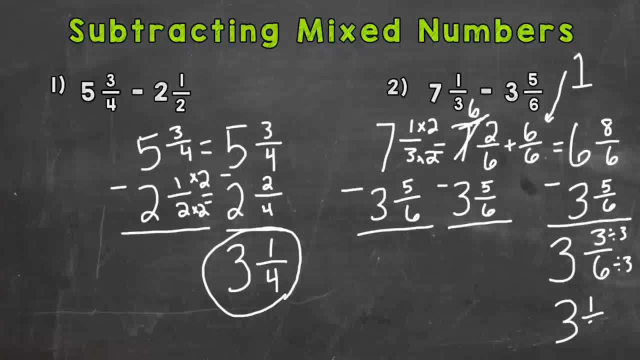 So this is how you subtract mixed numbers, And this actually turns out to be three and a half. That would be our final answer there. So there you have it. There's how you subtract mixed numbers. Rewrite the problem vertically. See if you need a common denominator, Rename. 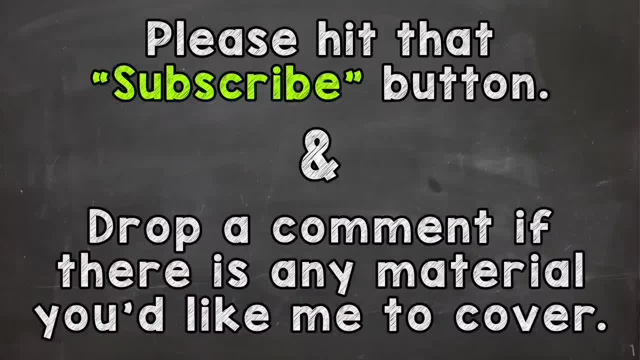